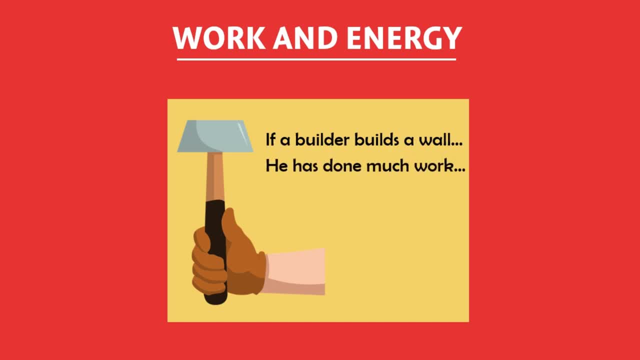 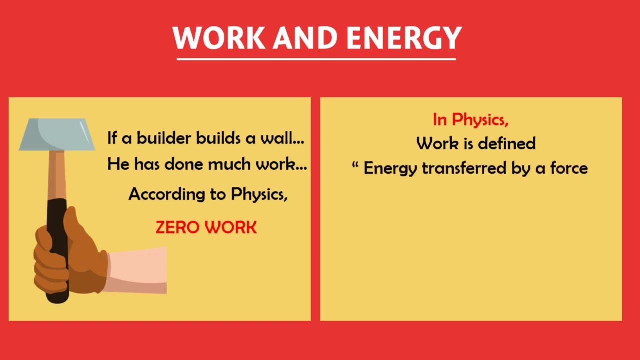 he may say after the day job that he has done much work, But in reality he has done zero work according to the physics rules. In physics, work is defined as the energy transferred by a force in its own direction. Or, to simple it, I can say that when you displace an object in the direction of your force. 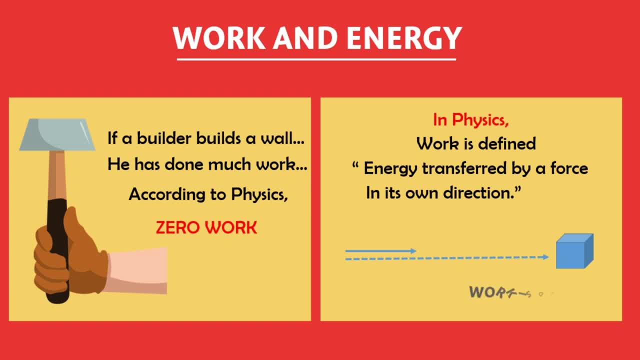 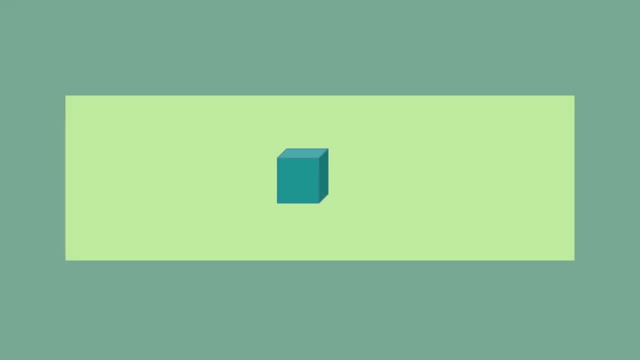 we say that, according to physics, you have done some sort of work. For example, if a block is present here, you exert force on this block in this direction and the block moves in the same direction, are in the direction of force. We can say that you have done work according to physics rule. 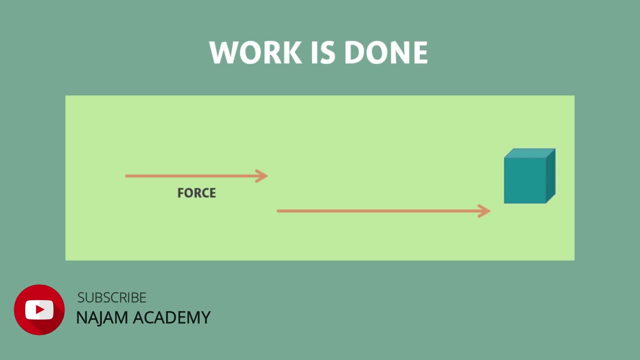 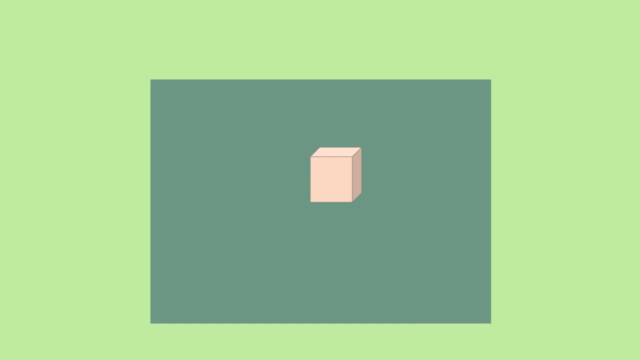 So remember this convention of physics, that whenever a force displaces an object in its own direction, we call this displacement of an object due to force as a work. Now, if another block is present here and you exert the force in this direction and the block moves in this direction, Can I say that you have done some sort of work on this object? 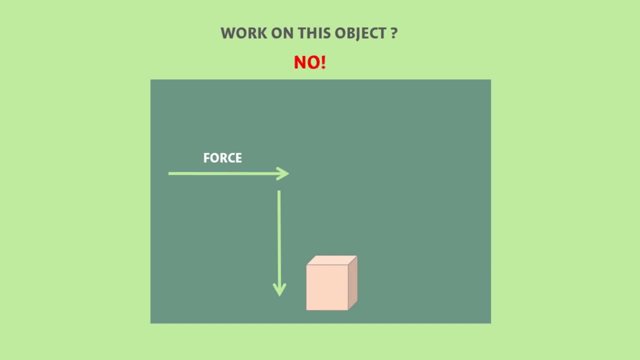 The answer is absolute. no One can say that I have exerted force on an object and the object is in the same direction And the object is displaced by my force. So, according to the definition, I have done some sort of work. But this is still wrong explanation. Here is the explanation that the work is zero. 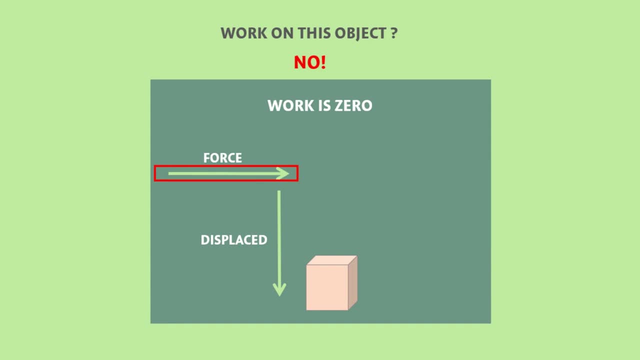 You have exerted force on this object in this direction, while the object is displaced in other direction. Hence the direction of my force and the direction of displacement of this object are not same. Hence work is zero here. Remember this simple rule that the direction of force and 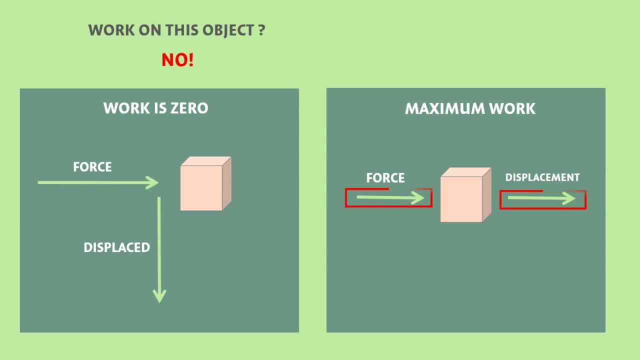 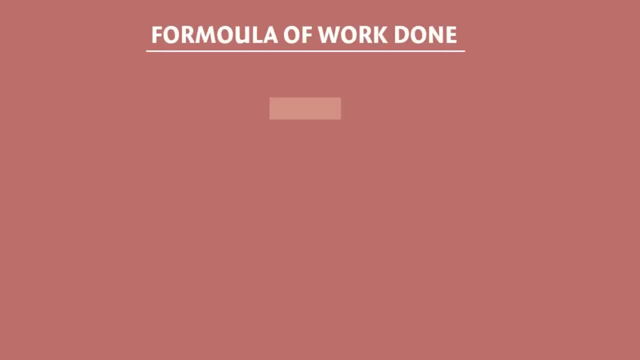 the direction of displacement should be same for maximum work done. Now let me discuss the formula of work. The formula of work done is equal to f dot d cos theta. If someone write f cross d cos theta, then this is the wrong formula, Because 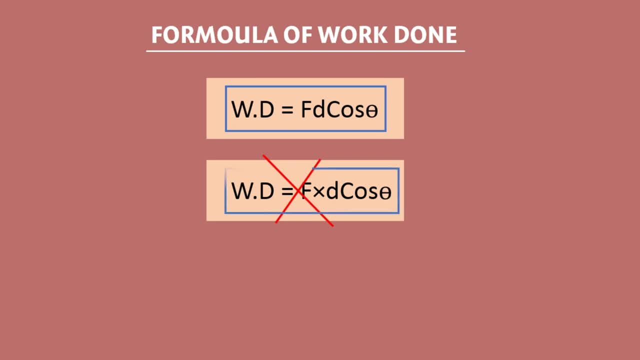 work done is a dot product. Work done is not a cross product. In this formula we already know that f is the force which we exert on an object and d is the displacement of an object and the direction of force. Then what about the cos theta? Well, the theta is the angle. 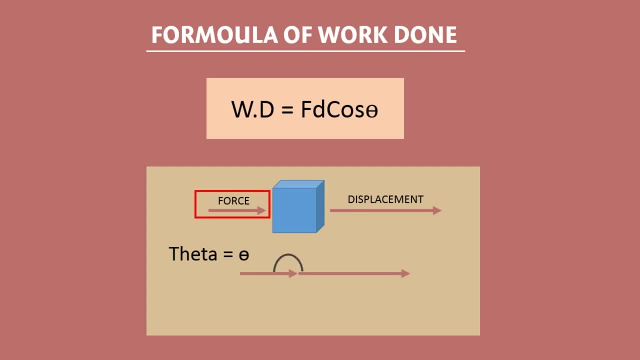 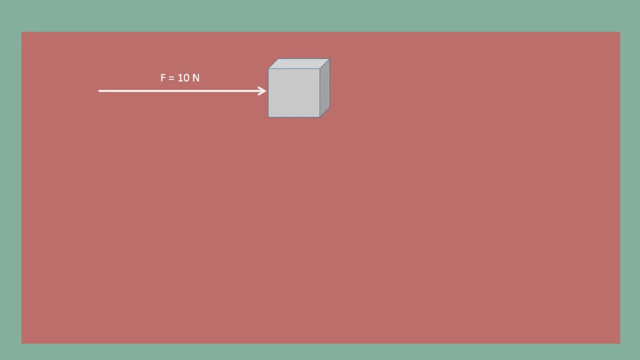 between the force which we exert on an object and the displacement of an object. Let me explain this work done formula by giving you some examples. If I put 10 Newton force on this object in this direction, then this object travels 20 meter in this direction. Here I know that the direction of force and the direction of displacement is same. 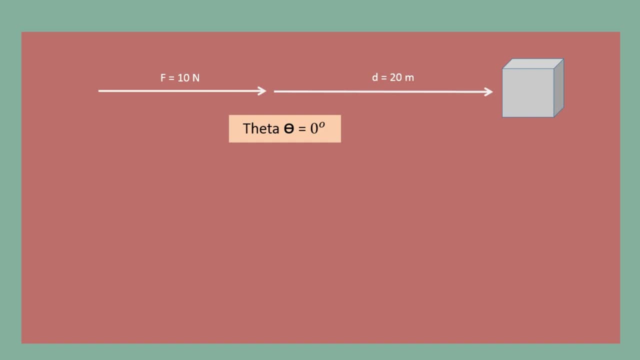 Hence the angle between them is zero. Therefore here theta is equal to zero degree. We already know that cos 0 degree is equal to 1.. I know the formula of Worden, which is equal to Worden, is equal to Fd cos theta. 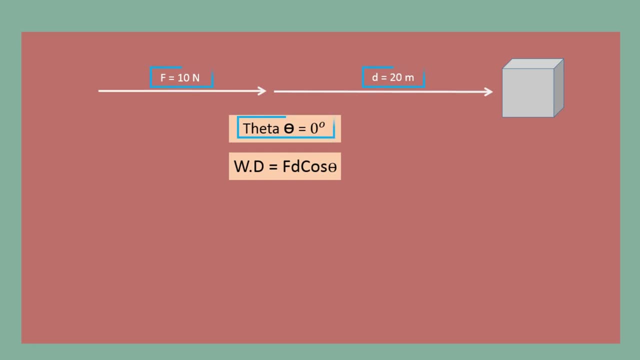 Hence putting values and the formula. Worden is equal to 10 N and to 20 m cos 0 degree, I get Worden is equal to 200 Nm. or I can say that Worden is equal to 200 J. Remember that there are two SI units of Worden. one is Nm and another is J. 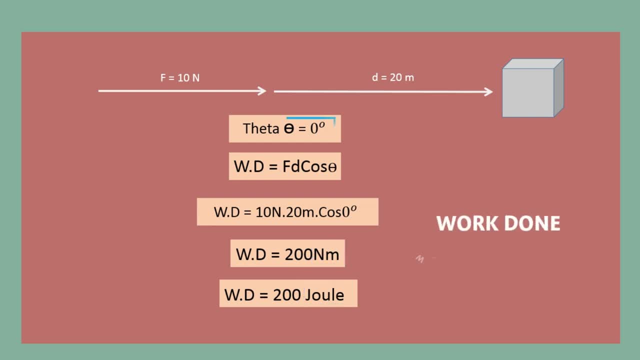 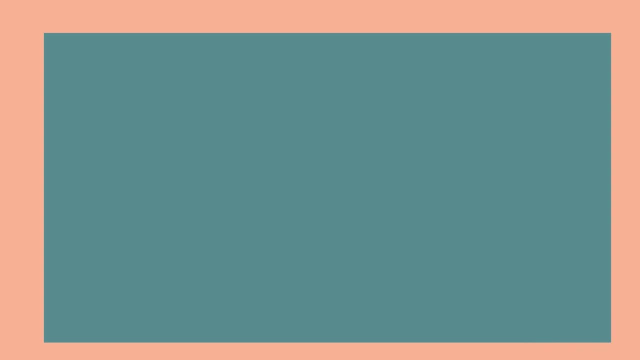 So in this example we learnt that Worden will be maximum if the angle between force and displacement is 0.. Let me give you another example. If you exert Fd 50 N force on an object and the object is displaced by 30 m in this direction, 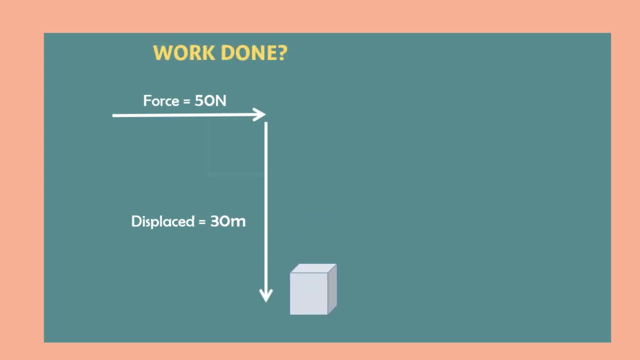 Then, what about the Worden? Well, here the angle between force and displacement is 90 degree, Hence theta is equal to 90 degree. Now, writing the formula of Worden Worden is equal to Fd. cos. theta Worden is equal to 50 N and to 30 N. 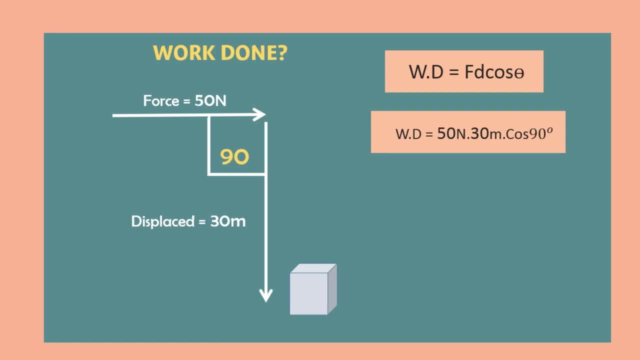 So in this example we learnt that when the angle between force and displacement is 90 degree, the Worden will be 0.. That's why I told you earlier in this lecture that when the direction of force and displacement is different, Worden will be 0. 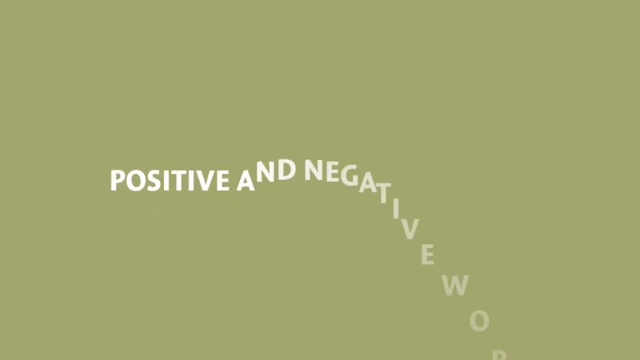 Let me also teach you the concept of positive work and negative work. First of all, remember that work is a scalar quantity. Therefore, work may be positive or negative. If you exert force on an object in this direction and the body moves in this direction, then 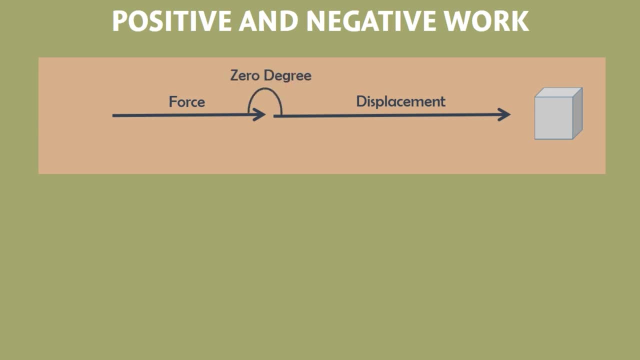 the angle between force and displacement is 0.. We also know that cos 0 degree is equal to 1.. Hence here Worden will be positive. On the other hand, if you exert a force on an object in this direction and the body moves, 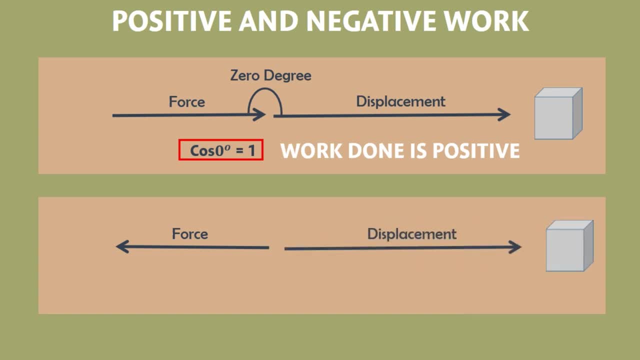 in this direction. here the angle between force and displacement is equal to 180 degree. We already know that cos 180 degree is equal to minus 1. Hence here 180 degree is positive. Hence here gravity will be negative. The negative sign indicates that if you exert a force in this direction, body will be displaced. 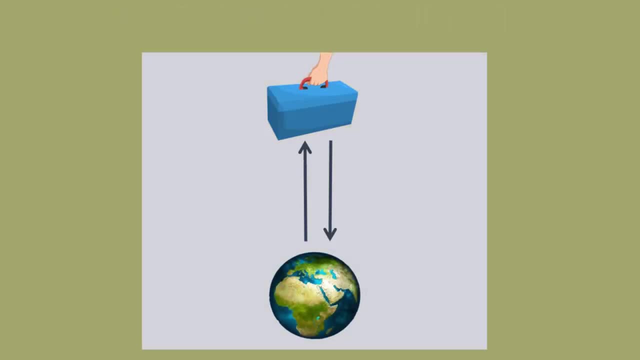 in opposite direction. In real life, when we raise an object from earth's surface, the displacement will be like this And the force of gravity will be in this direction. Hence the Worden against gravity will be negative. Now let me teach you about this. 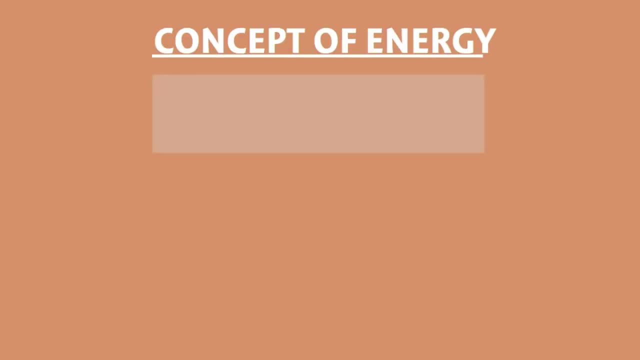 So let's start about the concept of energy. Energy is explained as the ability to do work, or the capacity to do work, As we learn that when we do some sort of work on an object, we displace the object from its mean or rest position. Or we can also say that when we do some sort of work on an object,